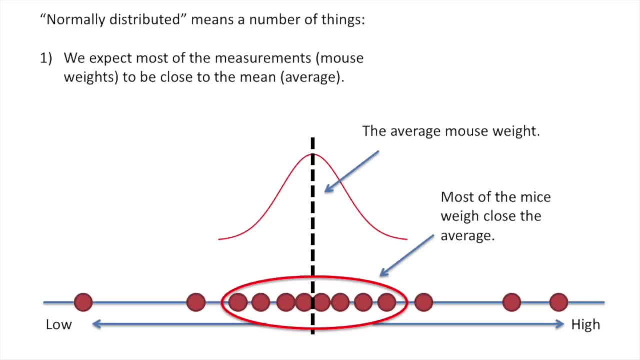 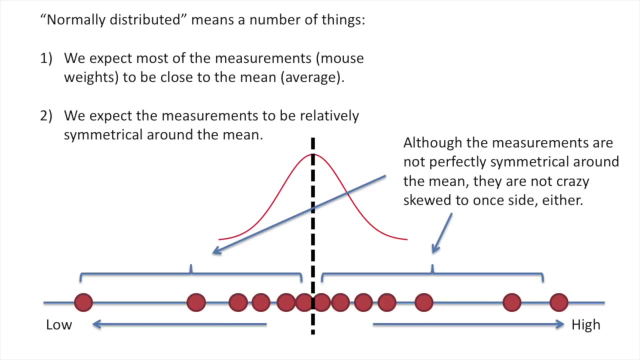 or average, And we see, lo and behold, in our data set, most of the mice weigh close to the average. We also expect the measurements to be relatively symmetrical around the mean. Although the measurements are not perfectly symmetrical around the mean, they are not crazy skewed to one side. 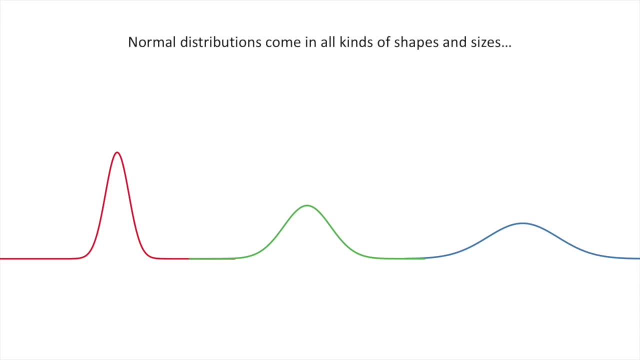 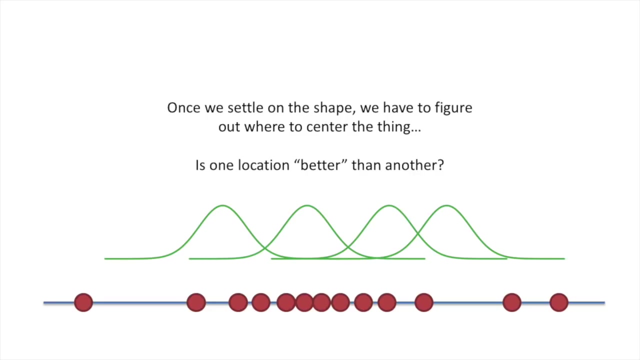 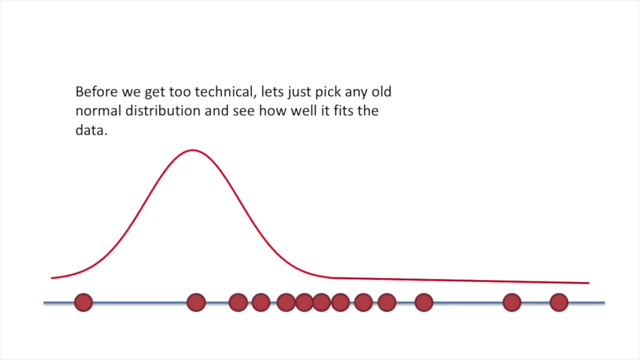 either. This is pretty good. Normal distributions come in all kinds of shapes and sizes. They can be skinny, medium or large boned. Once we settle on the shape, we have to figure out where to center the thing. Is one location better than another? Before we get too technical, let's just pick any old normal. 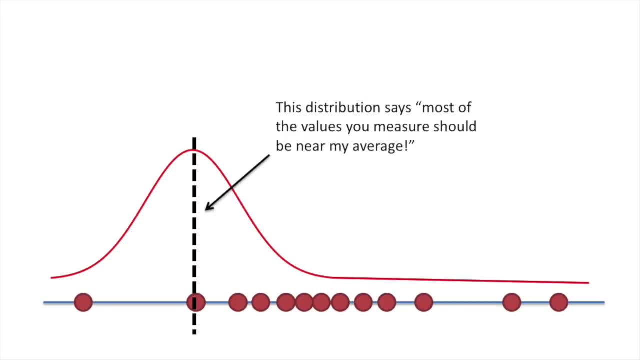 distribution and see how well it fits the data. This distribution says most of the values you measure should be near my average. The distribution's average is the black dotted line. In this case that's different from the average of the actual measurements. 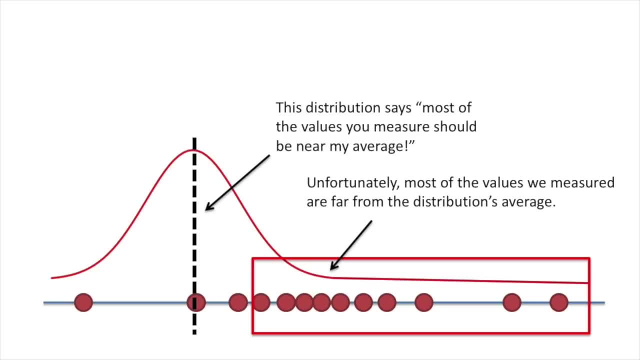 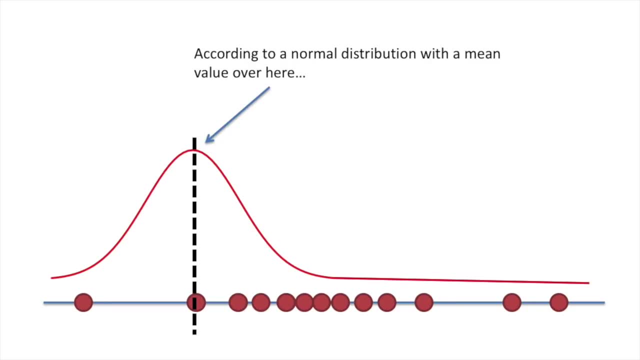 Unfortunately, most of the values we measured are far from the distribution's average. According to a normal distribution with a mean value over here, the probability or likelihood of observing all these weights is low. What if we shifted the normal distribution over so that its mean was the same as the average weight? 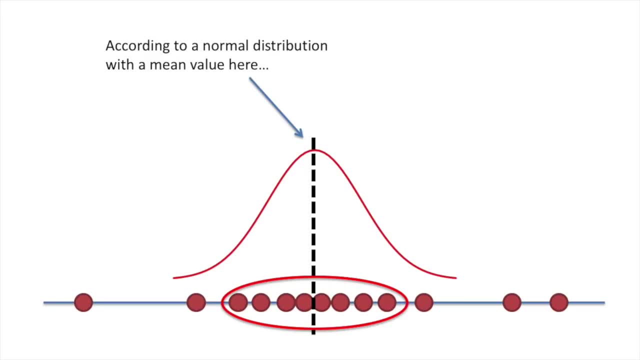 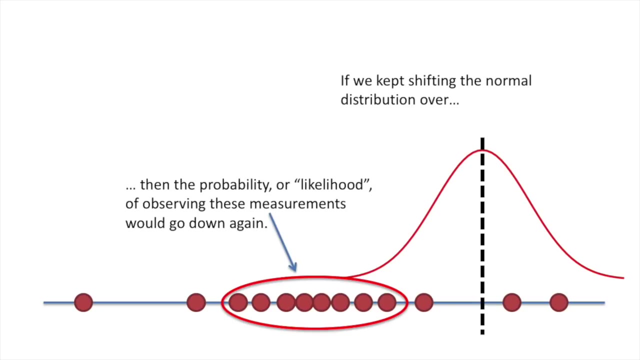 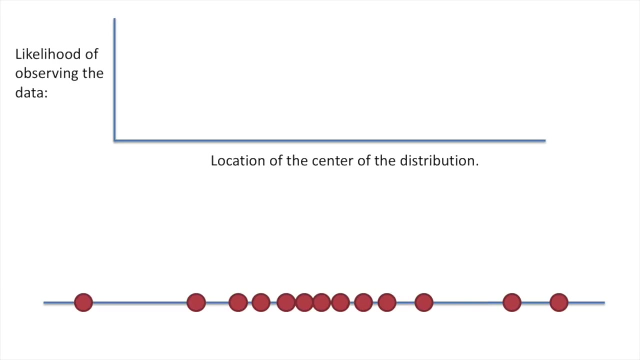 According to a normal distribution with a mean value here, the probability or likelihood of observing these weights is relatively high. If we kept shifting the normal distribution over, then the probability or likelihood of observing these measurements would go down again. We can plot the likelihood of observing the data over the location of the center of the. 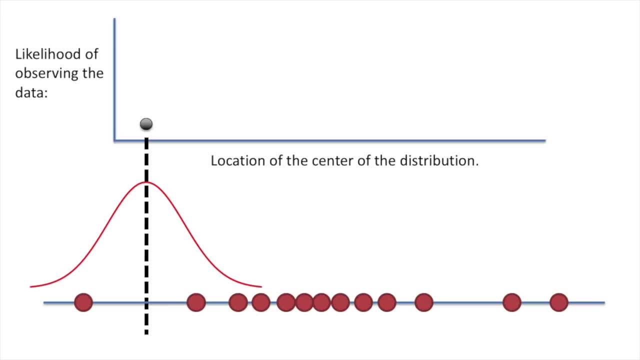 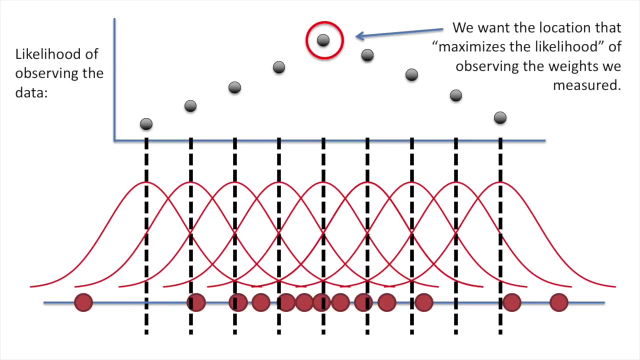 distribution. We start on the left side and we calculate the likelihood of observing the data and then we shift the distribution to the right and recalculate. we just do this all the way down the data. Once we've tried all the possible locations, we could center the normal distribution. 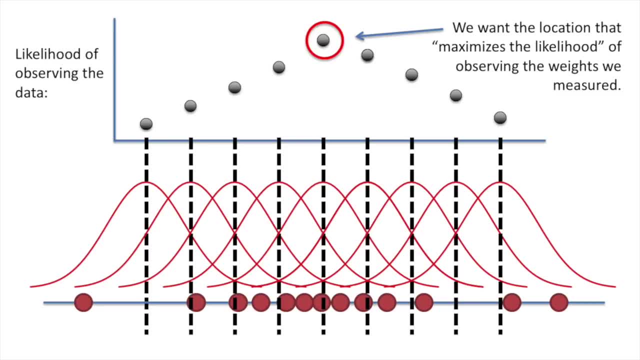 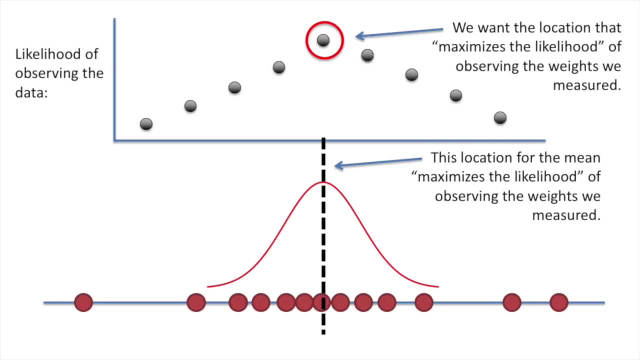 on. we want the location that maximizes the likelihood of observing the weight weights we measured. This location for the mean maximizes the likelihood of observing the weights we measured. Thus, it is the maximum likelihood estimate for the mean. In this case, we're specifically talking about the mean of the distribution, not the mean of. 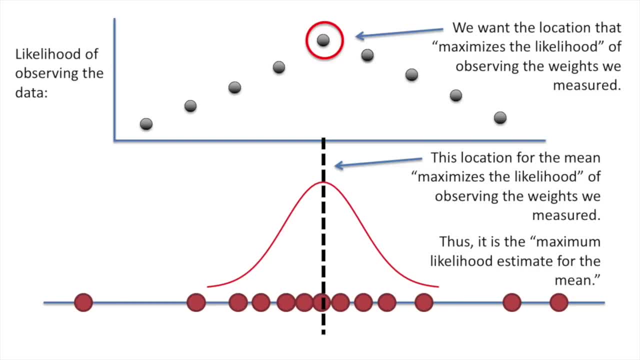 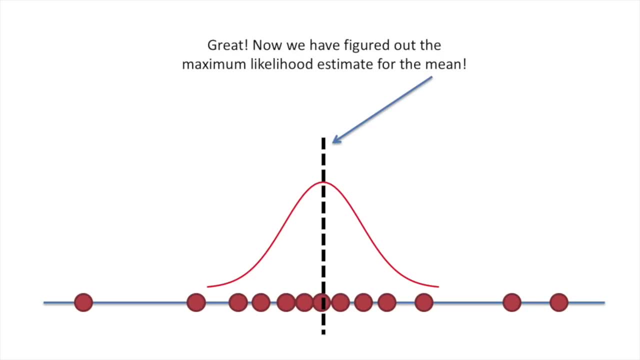 the data. However, with a normal distribution, those two things are the same, Great. Now we have figured out the maximum likelihood estimate for the mean. Now we have to figure out the maximum likelihood estimate for the standard deviation. Again, we can plot the. 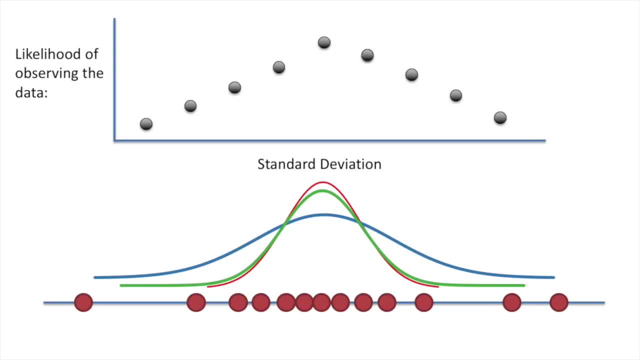 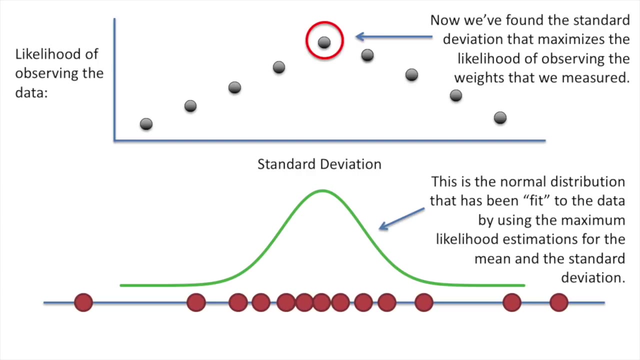 likelihood of observing the data over different values for the standard deviation. Now we found the standard deviation that maximizes the likelihood of observing the weights we measured. This is the normal distribution that has been fit to the data by using the maximum likelihood estimate for the standard deviation. 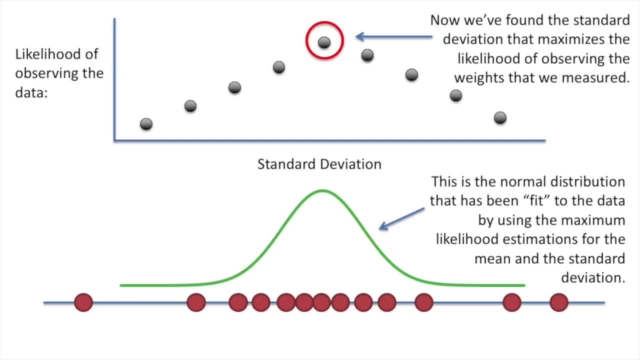 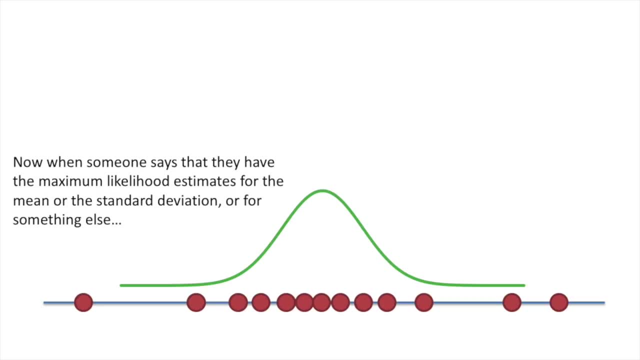 maximum likelihood estimations for the mean and the standard deviation. Now, when someone says that they have the maximum likelihood estimates for the mean or the standard deviation or for something else, you know that they found the value for the mean or the standard deviation. 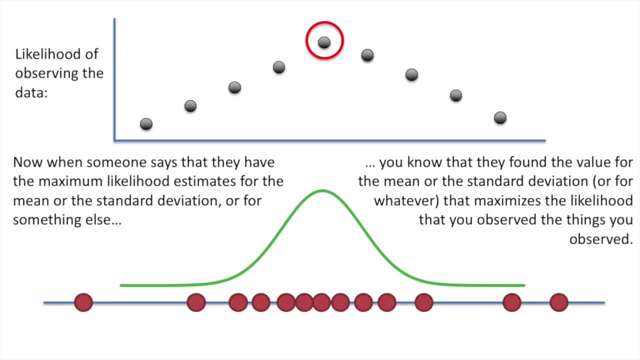 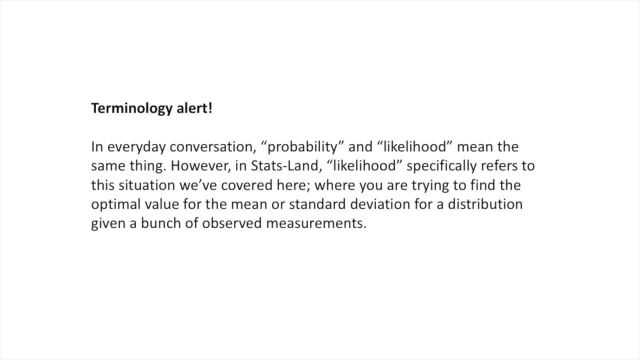 or for whatever that maximizes the likelihood that you observed the things that you observed. Terminology Alert: In everyday conversation, probability and likelihood mean the same thing. However, in Stats, Land likelihood specifically refers to this situation we've covered here, where you are trying to find the optimal value for the mean or standard deviation. 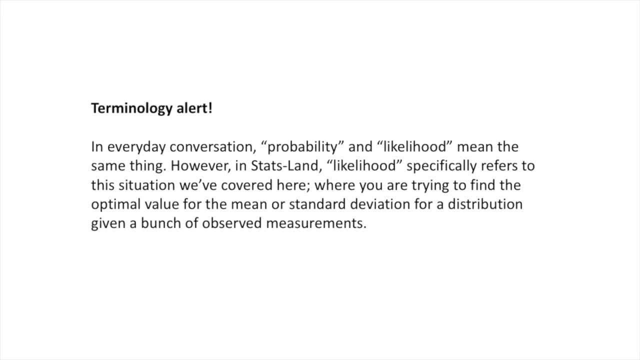 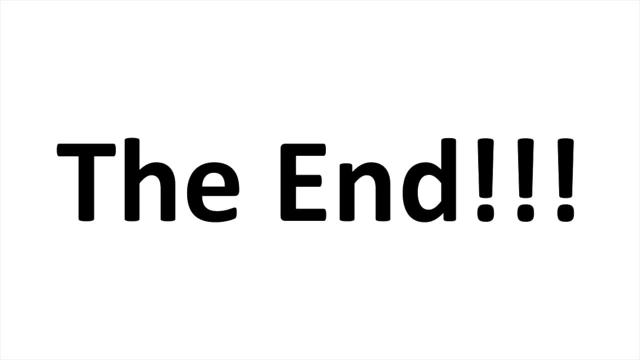 for a distribution given a bunch of observed measurements. This is how we fit a distribution to data. Hooray, We've made it to the end. We've made it to the end of another exciting StatQuest. If you like this StatQuest and want to see more like it, 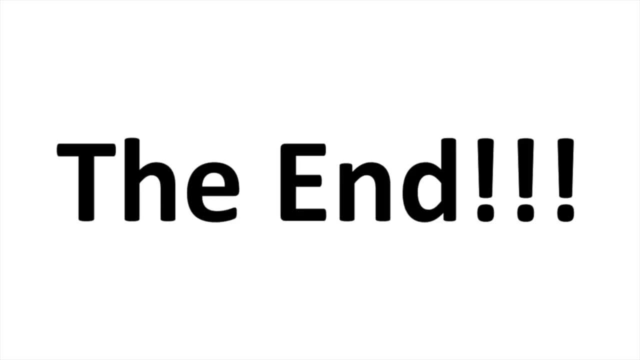 please subscribe. It's super easy. Just click the little button below And if you have any suggestions for other StatQuests that I could do, put them in the comments. Alright, until next time. Quest on.